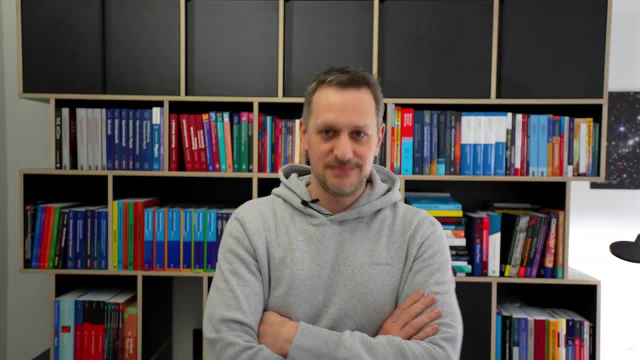 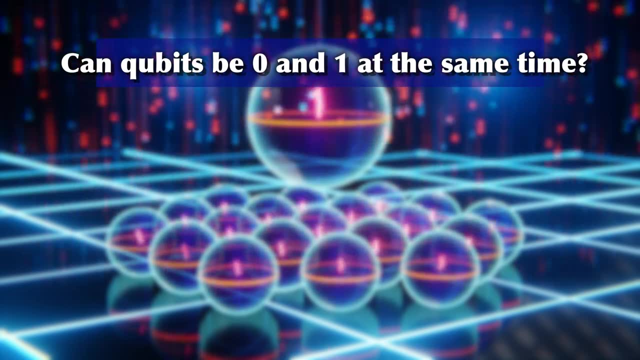 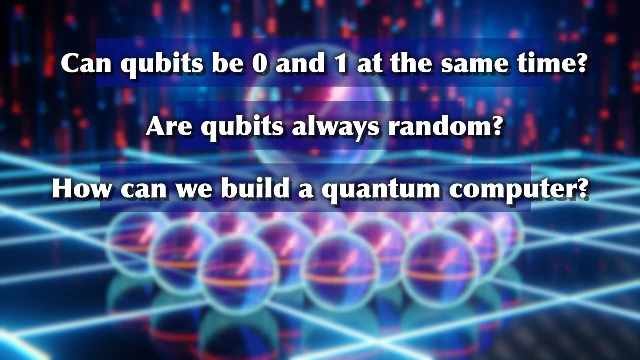 This would also allow me to go to a much deeper explanation. That way, we can talk in a much more meaningful way about questions like: Is it true that qubits can be zero and one at the same time? Are they always random, And if so, how can we build a useful computer around that? 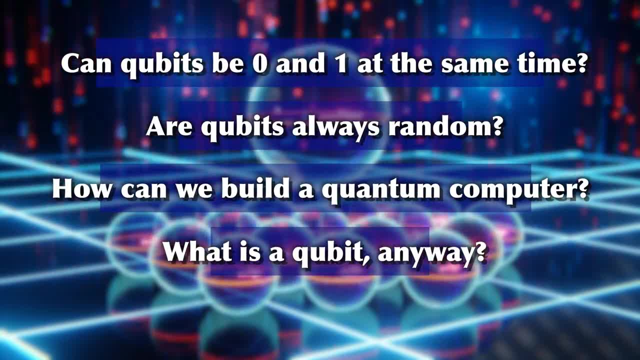 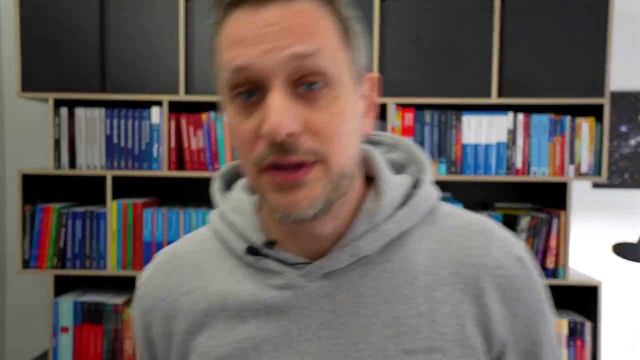 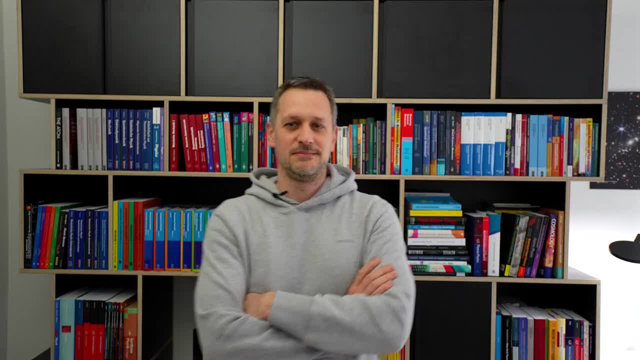 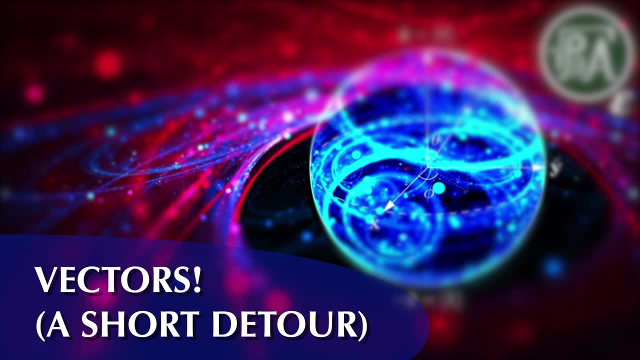 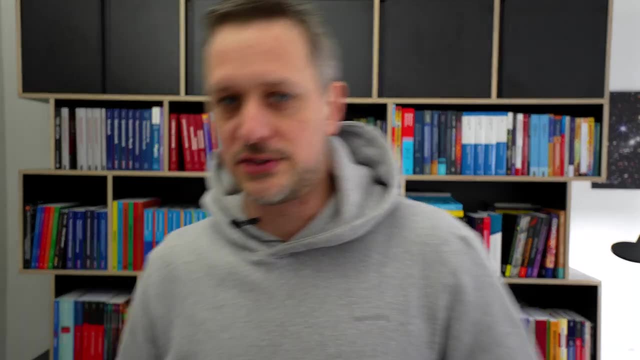 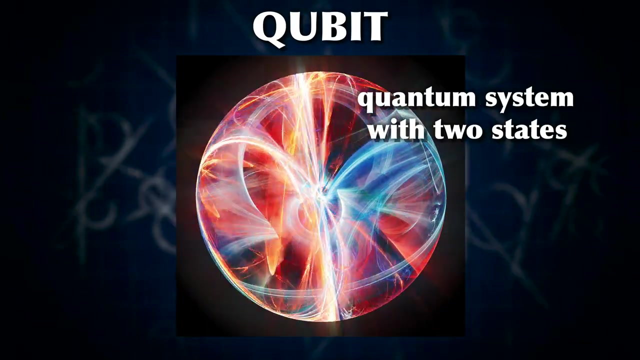 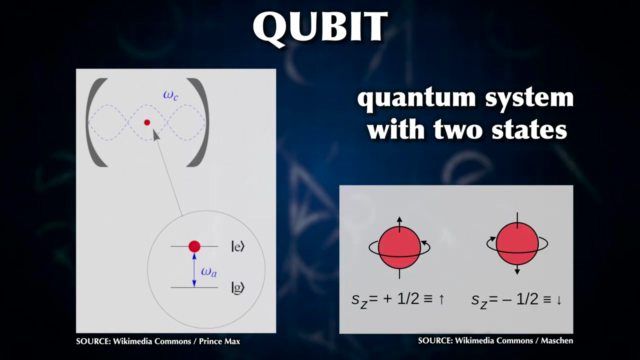 Ready, Let's go. Let's start with the obvious first question: What is a qubit? What is is a quantum mechanical system that has two different states. it can be in, for example, two different energy levels in an atom or ion, or two different spin states of a photon or electron. 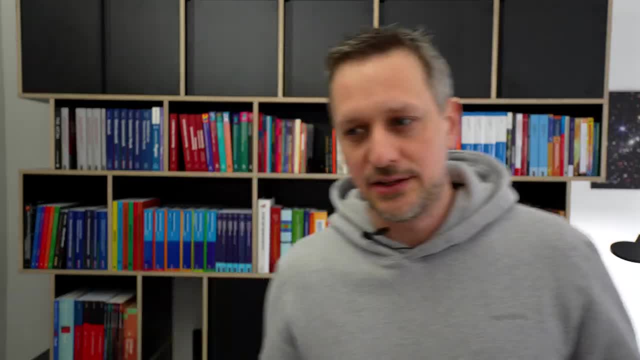 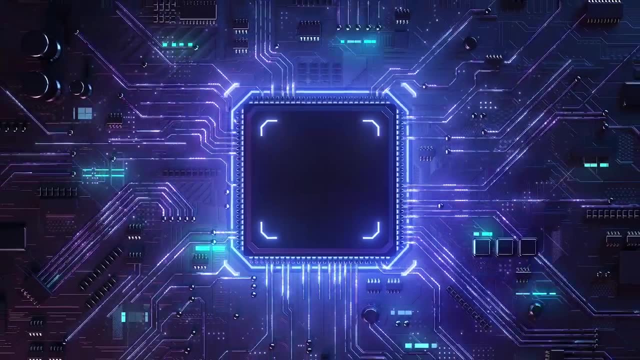 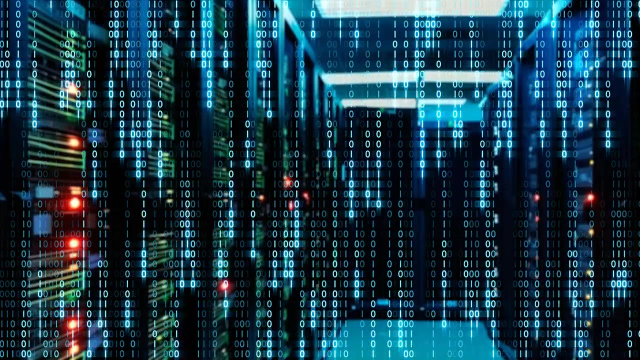 Anyway, the beauty of quantum computing is that we do not even have to understand all the details of the underlying physical system. Just like with normal digital computing, you do not need to understand all the details of voltage and current and all the electrical signaling. All you need to. 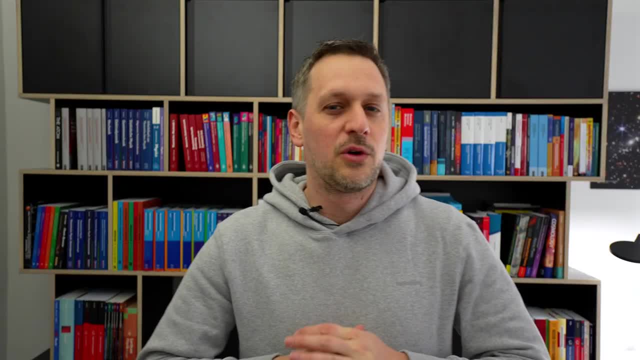 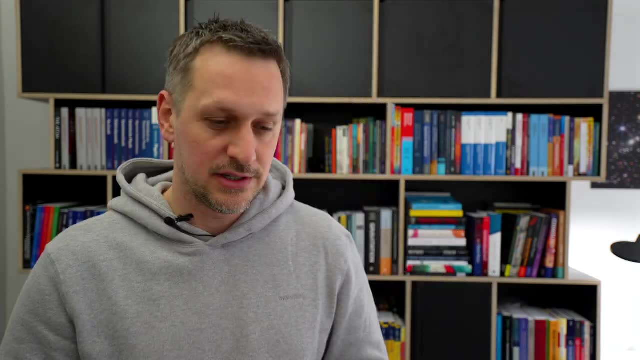 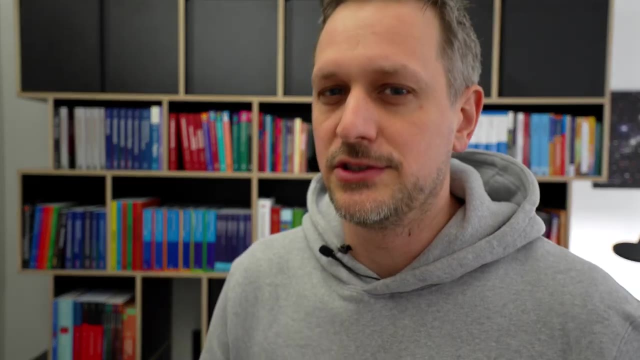 know is there's zeros and there's ones For quantum computing. all we need to understand is there is a system that is small and isolated enough to be quantum in nature and it has two states: zero and one. In other words, qubits are inherently two-dimensional, and to model this, 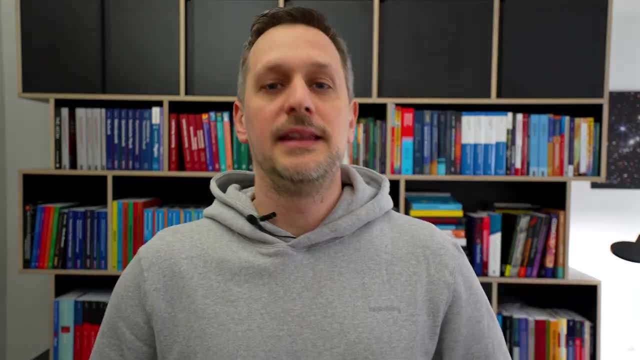 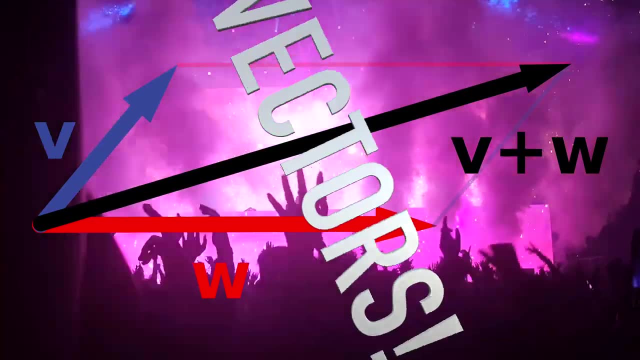 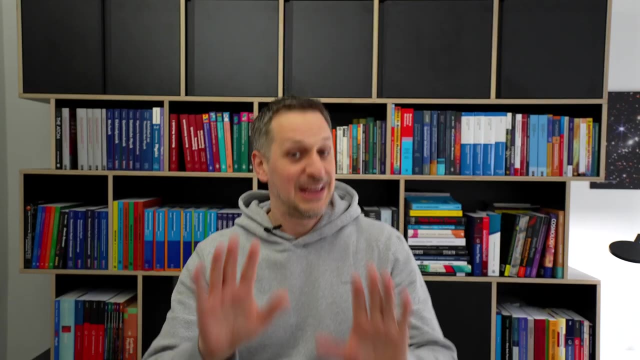 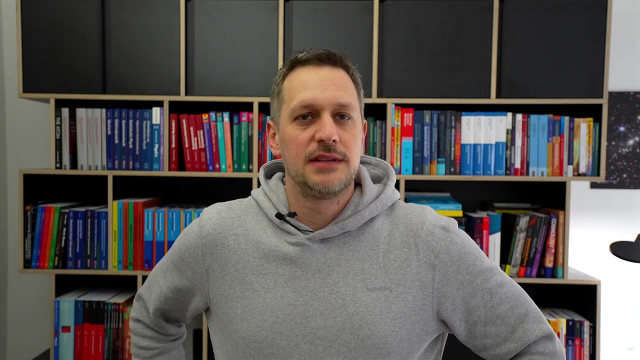 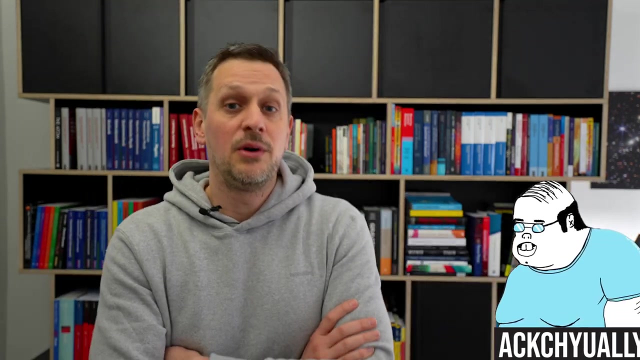 correctly. we need to take some ideas of a field called linear algebra. That's right. vectors, Okay, okay. okay, stay with me. this will make much more sense in a minute. In the most basic sense, a vector simply denotes direction. Of course, the concepts of vectors and vector spaces are far more. 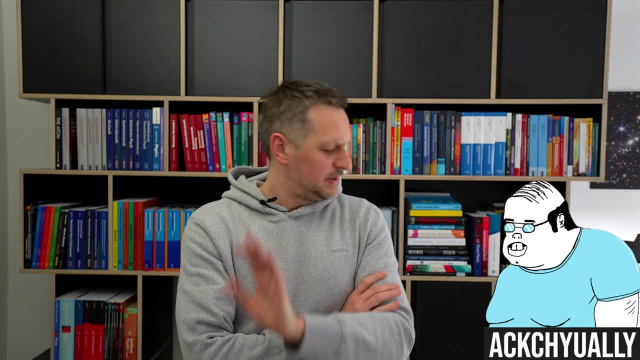 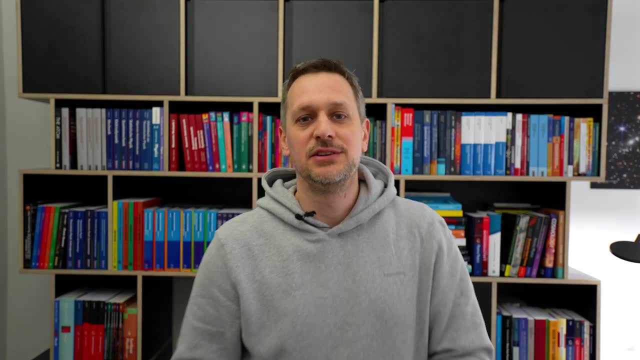 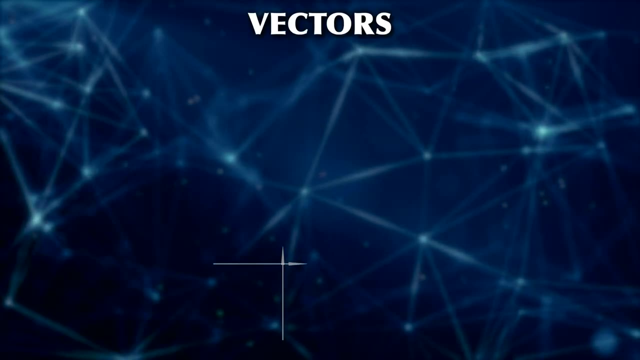 abstract and comprehensive than that, But we simply do not need this here, Right? so, as I said, directions To define a geometrical vector. we simply say it goes from here to here and then we draw it as an arrow. For example, in 2D space we can have a vector in the x-direction or the y-direction. We usually 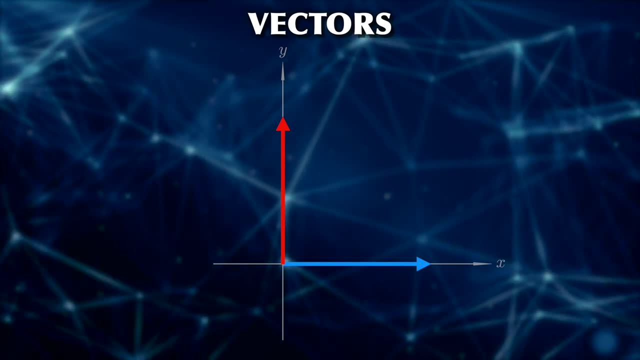 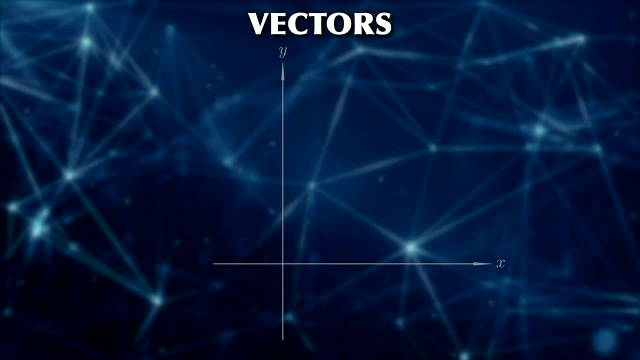 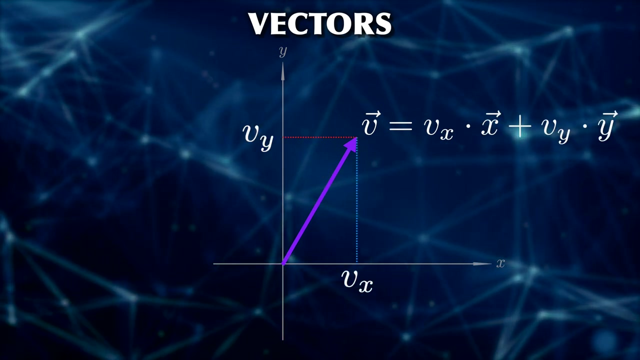 signify vectors by a little vector arrow so we can write. This arrow is just a symbol that tells us that something is a vector. We can also have a vector in an intermediate direction, meaning it has a vector in the x-direction and another component in the y-direction. Another important thing is: 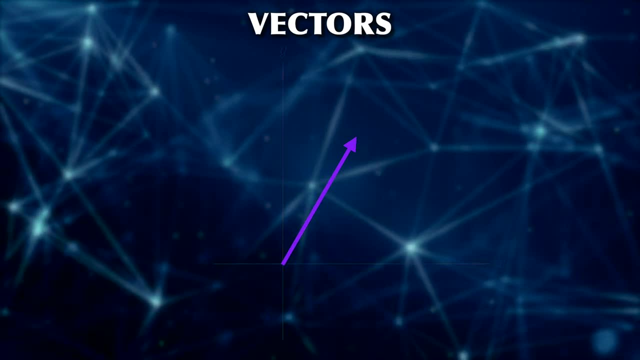 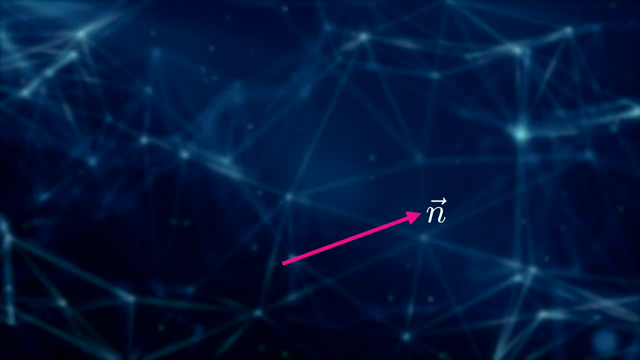 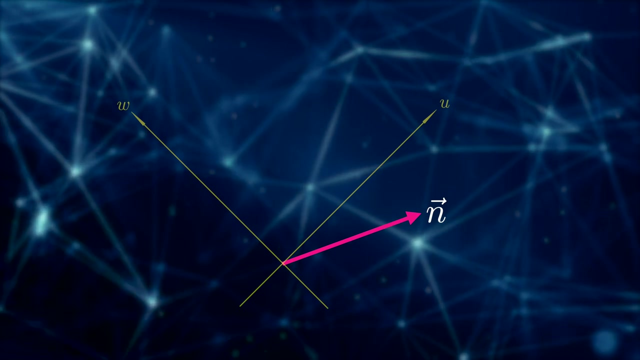 that we do not have to use x and y to describe vectors. We can use a different basis, For example, two different vectors: u and w. We can describe any vector in either the x and y basis or the u and w basis, or any other basis that we choose. Okay, that's all we need. Let's go back to bits and qubits. 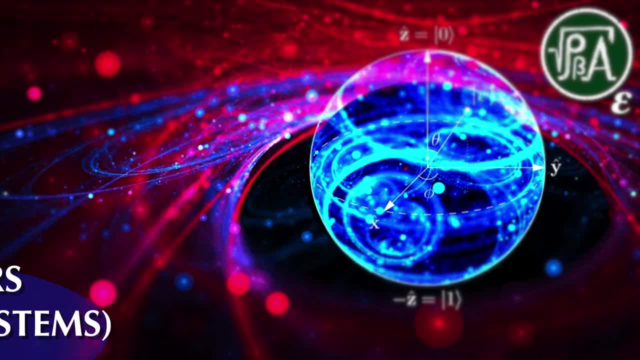 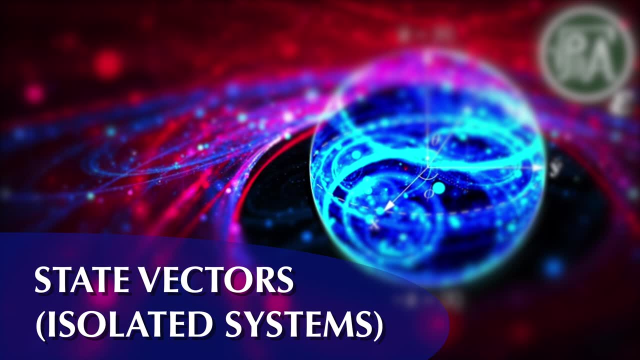 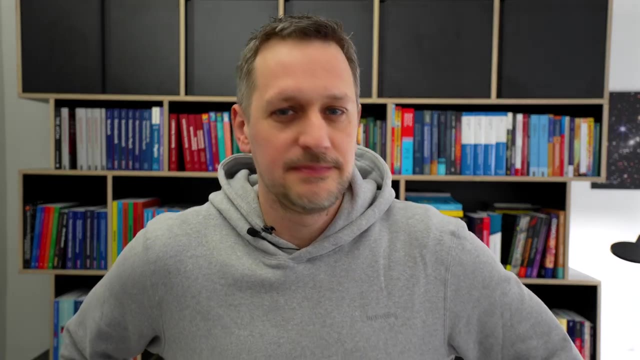 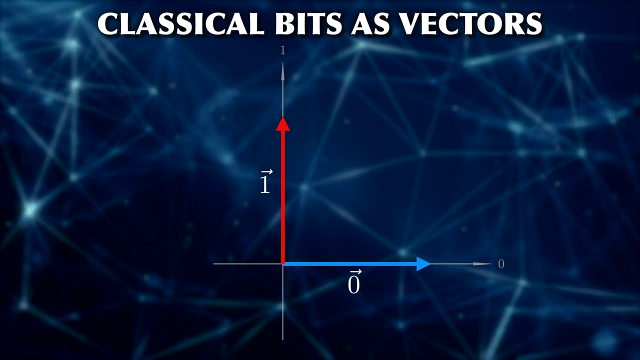 The connection between vectors and bits and qubits is this: Classical bits are much like two separate directions, For example the x and y vectors. But this is such a simple system that we usually do not even bother with the vector description, because we would not be able to describe the vector in this way. 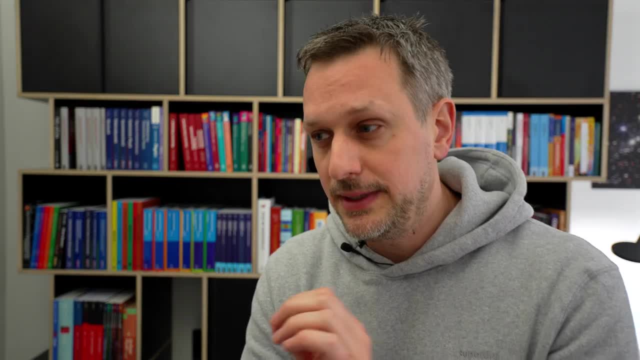 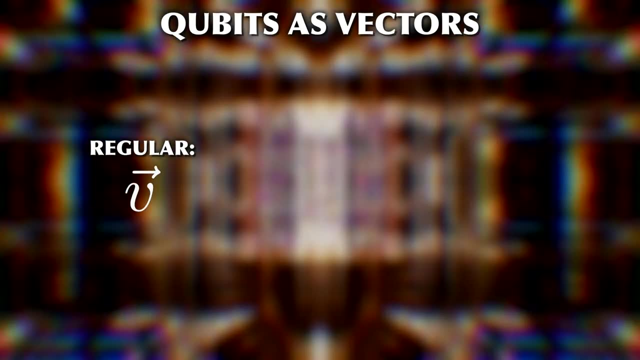 We would gain very little from it. Qubits, though, can be in any mixture of states, so the vector description is both useful and meaningful. You may have seen this before. In quantum physics, we use a slightly different notation for vectors, called the Dirac notation. 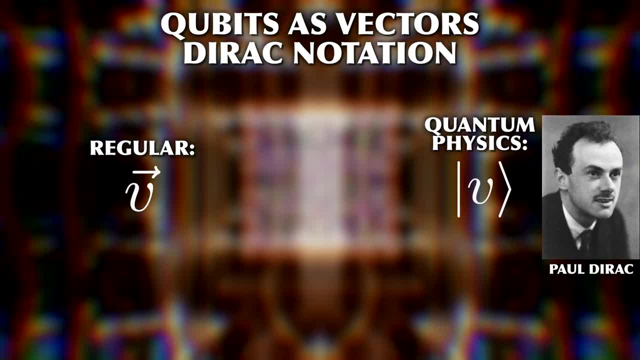 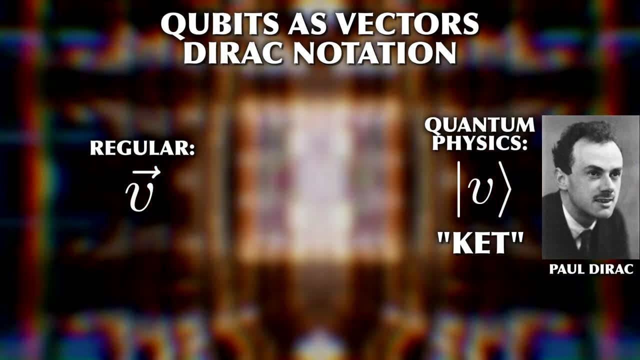 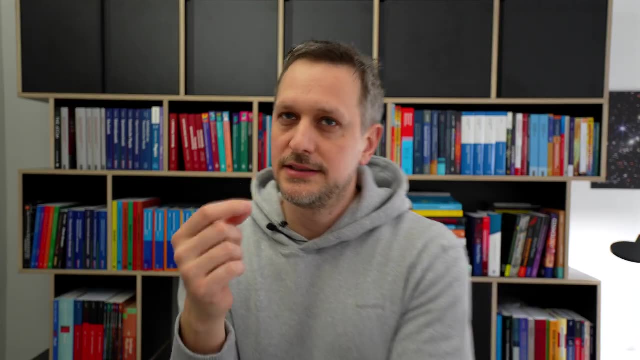 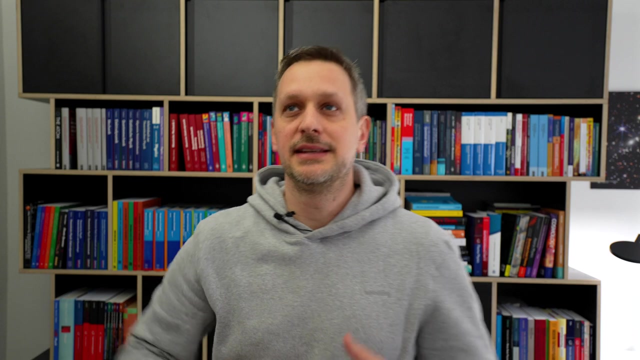 We write a state vector like this and call it a cat for quote silly reasons. Note that this is not a geometrical vector which gives a a real direction in real space. It's a vector of an abstract state space where the directions are equal to the states the system can be in. 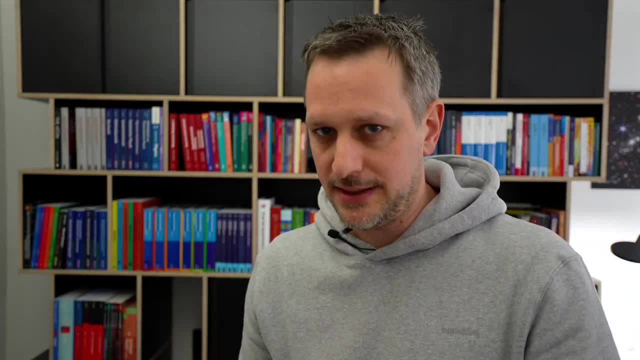 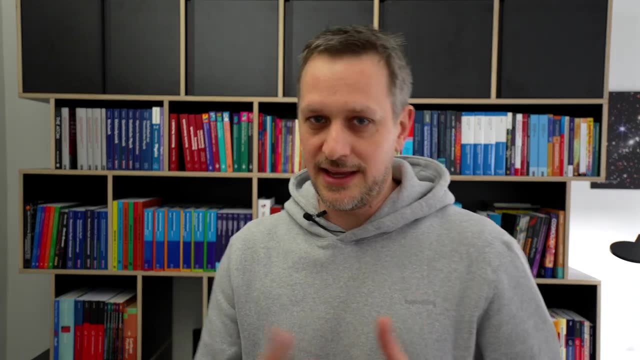 So the direction of the state vector indicates which mixture of states the qubit is in. According to the rules of quantum mechanics, a general state of a two level system is a general state of the system. So what's the general state of a quantum system? 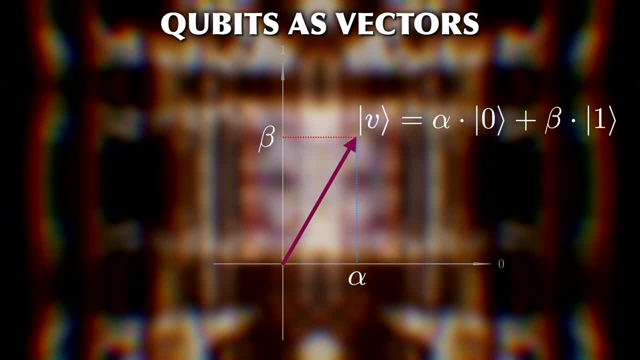 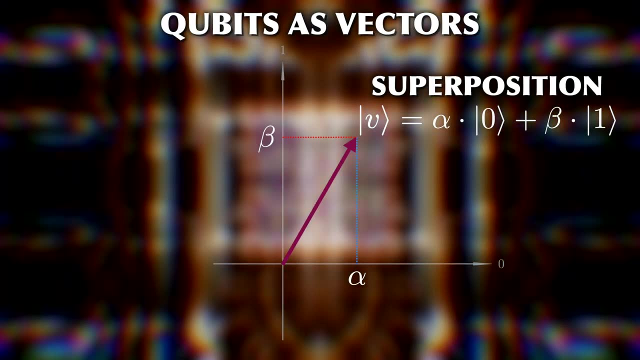 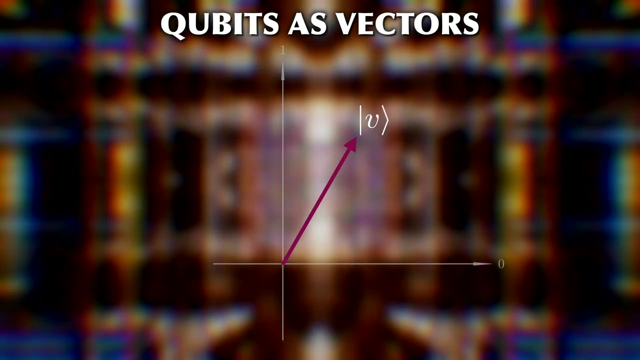 system like a qubit can be written like this More precisely, we say that the qubit is in a superposition of the state 0 and 1 and alpha and beta are the respective amplitudes. In the case of qubits we have the standard basis of 0. 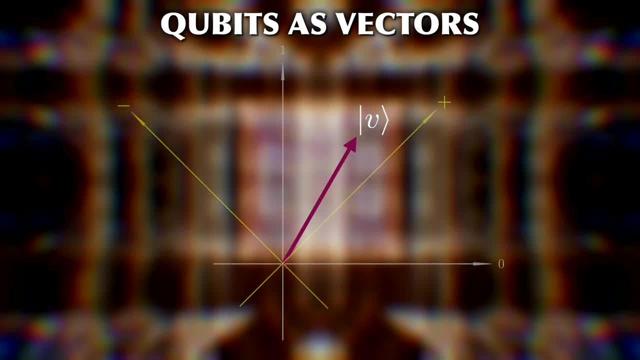 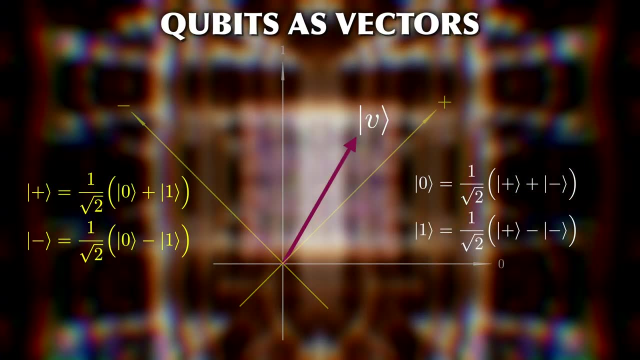 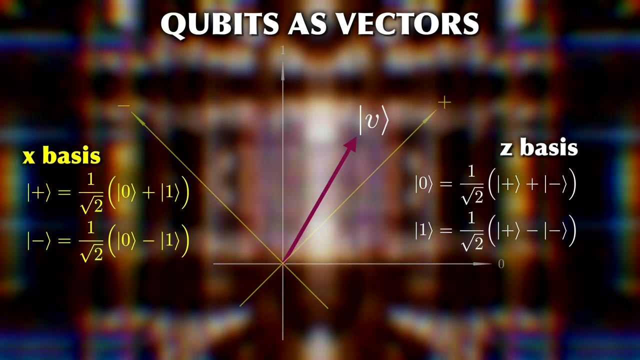 and 1, but we can also use the plus and minus basis. These two bases are related and can be freely transformed from one to the other. For historical reasons we call these the c-basis and x-basis. One other important consequence: we can 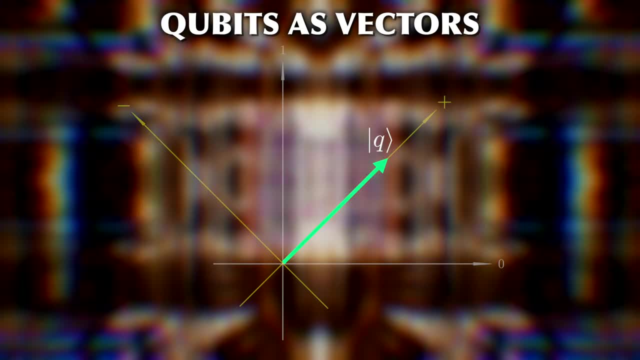 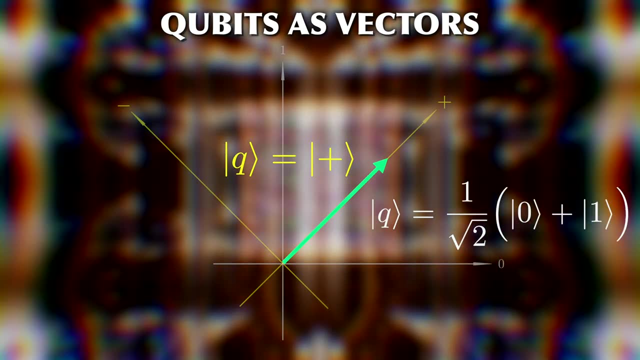 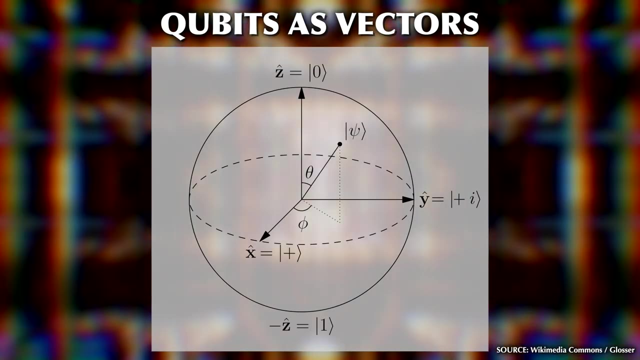 immediately see here is that if you describe a state in a different basis, the superposition may vanish. So whether state is in a superposition or not is entirely dependent on the basis used. We can go a step further and define a third dimension for the qubit, called the. 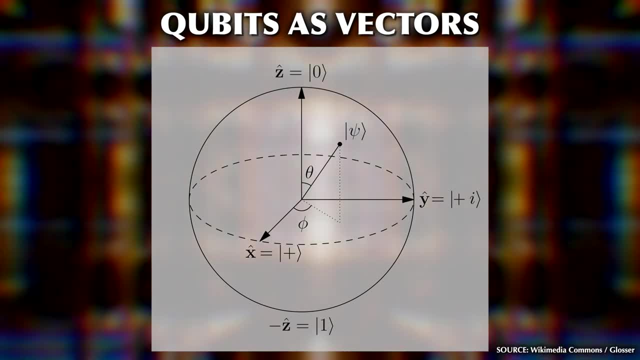 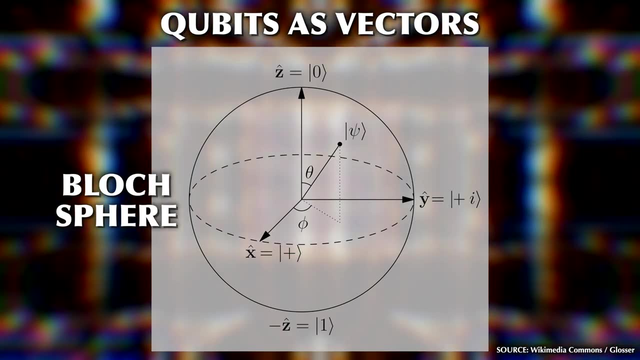 plus i and minus i states. and if we adjust the angles in this diagram a bit, this gives us the so-called Bloch sphere, A common and useful depiction of single qubits. Either way, state description is only one half of the quantum weirdness. 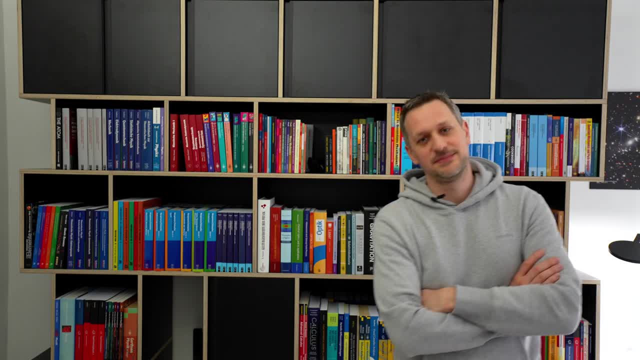 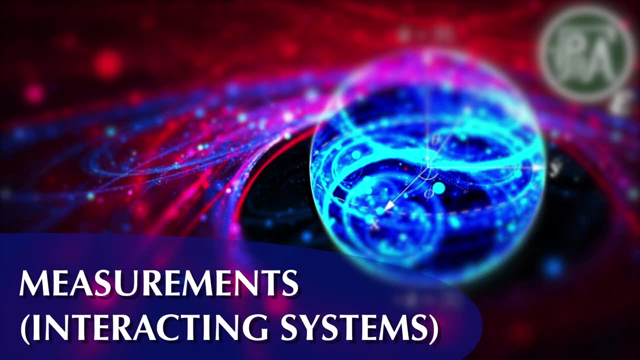 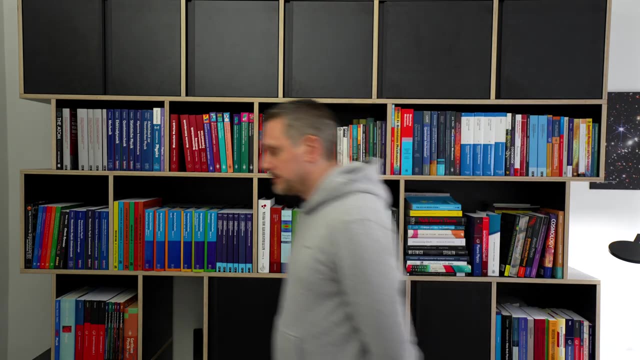 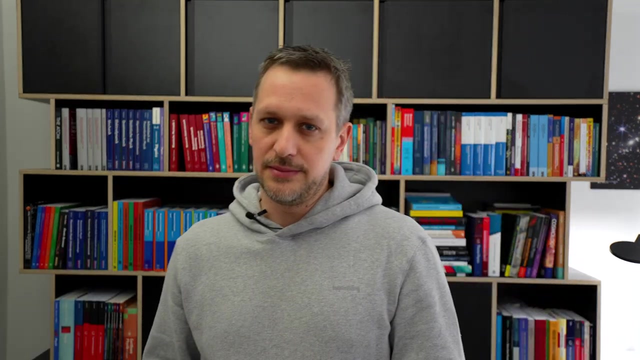 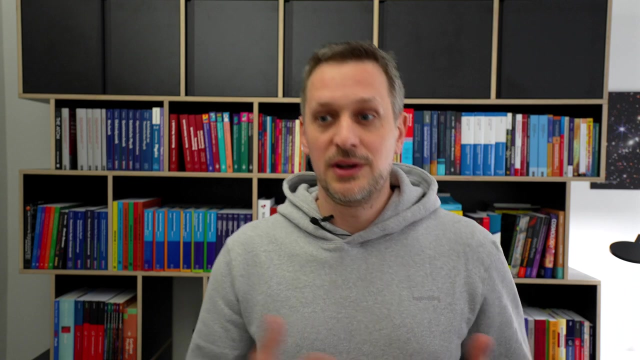 The second half is measurement. Everything I've said about quantum states so far only applies to isolated systems, So systems that do not interact with their environment. However, the entire point of computation is to generate some output, So sooner or later you will have to make a measurement and an interaction with the system, And these are the 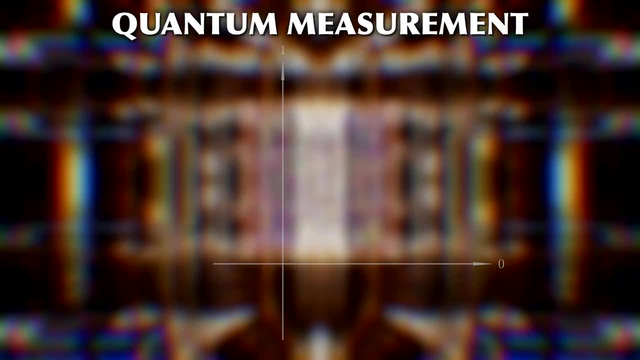 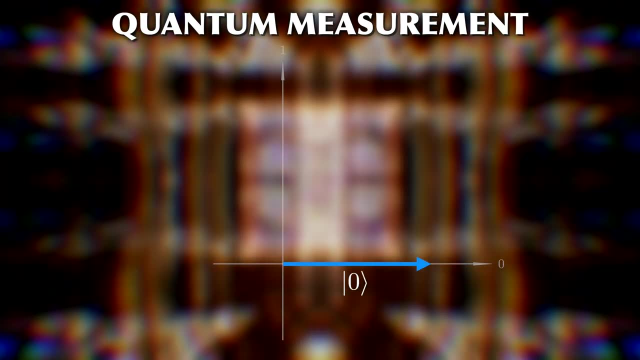 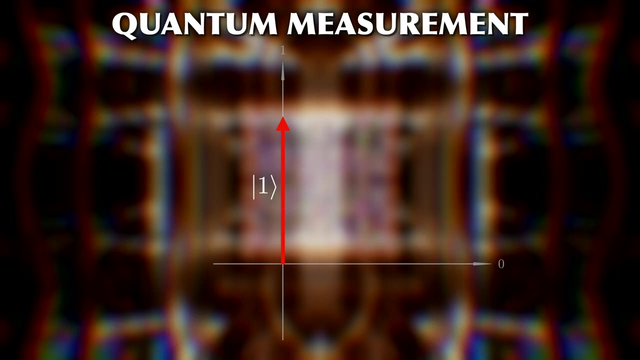 rules for measurements. Whenever you perform a measurement, the qubit is forced into one of the possible basis states. So you can only ever measure zero or one, Never both. So even if you can potentially encode more information in qubits, you can only ever get one bit of information out. This projection onto a 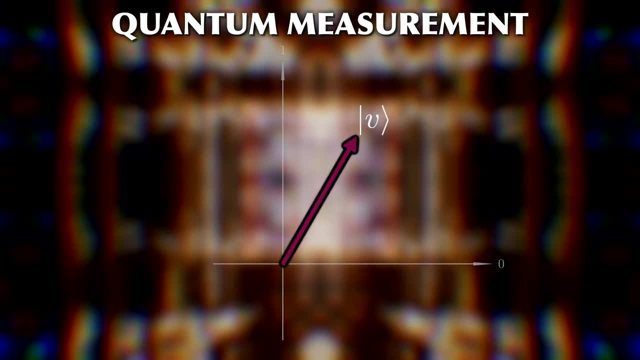 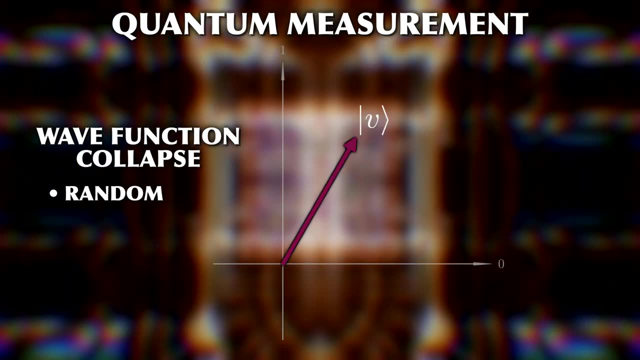 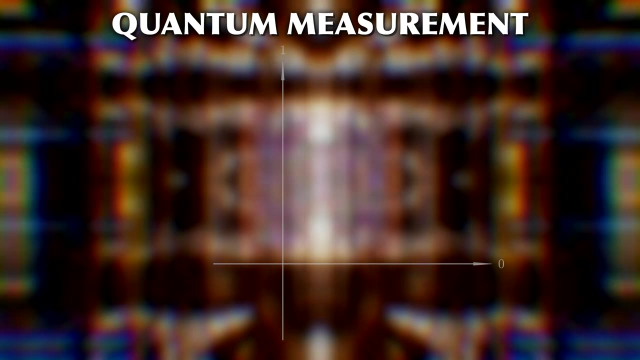 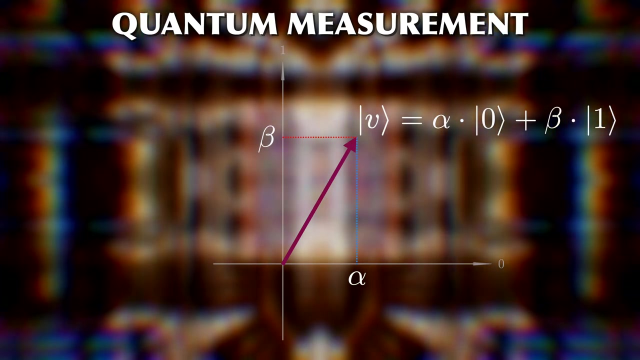 basis state triggered by measurement is called state reduction or the collapse of the wave function And, as far as we can tell, it is random, irreversible and almost instantaneous. While the measurement result is random, the meaning of a superposition is that the amplitudes give the probabilities for 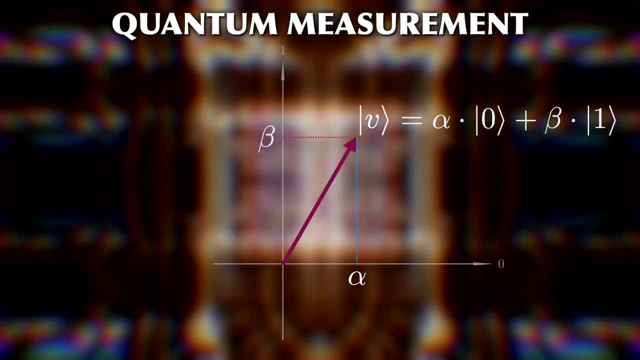 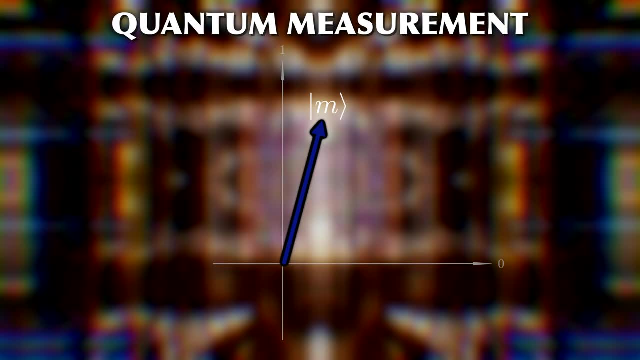 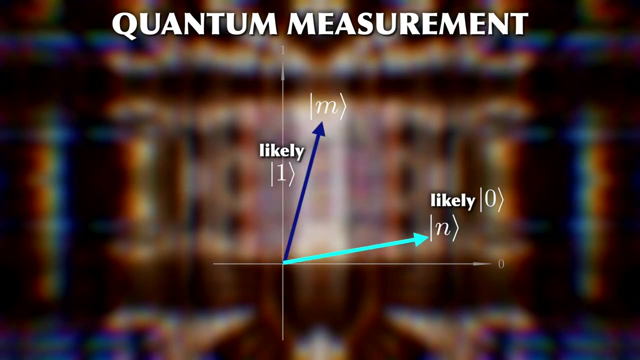 the different results. The state with the larger amplitude is more likely to be the outcome In terms of our vector language. if the state vector points more in the direction of one basis state, then this state is more likely to be measured. This also means that if a state already is in a basis state, you will get that result. 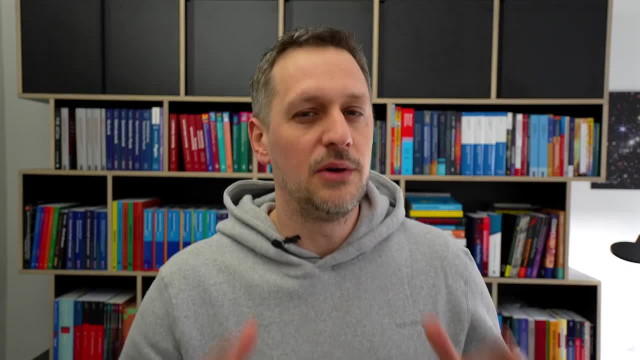 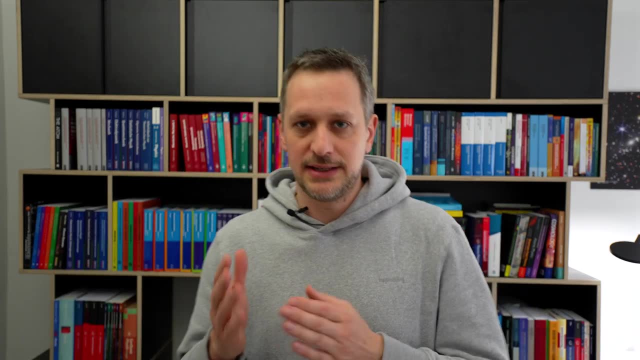 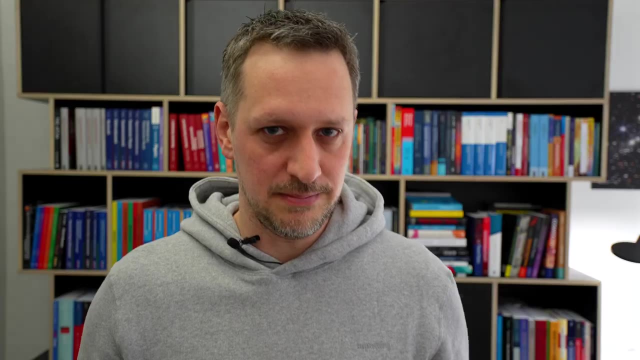 with one hundred percent probability. So if you have many identical copies of a quantum state, you can predict the distribution of the measurement outcomes. But each individual measurement will be random and you can only give the probability for each outcome. Also, any measurement can only be performed in a specific basis If you 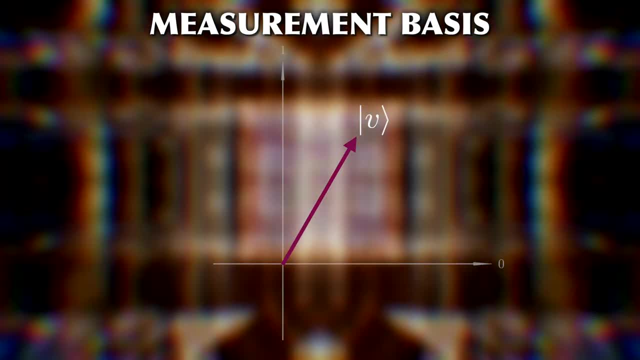 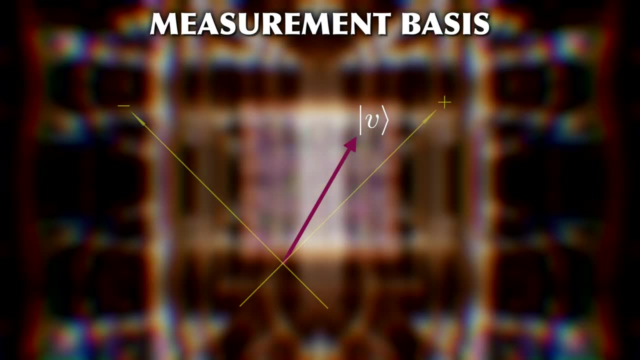 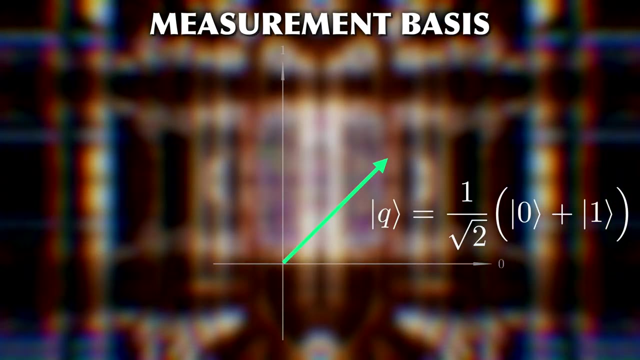 measure a qubit in a C basis, you only get the zero or one status outcome. Well, when you measure it in the X basis, you can only get the plus or minus states, etc. Let's look at an example: The state one over square root of two times zero. 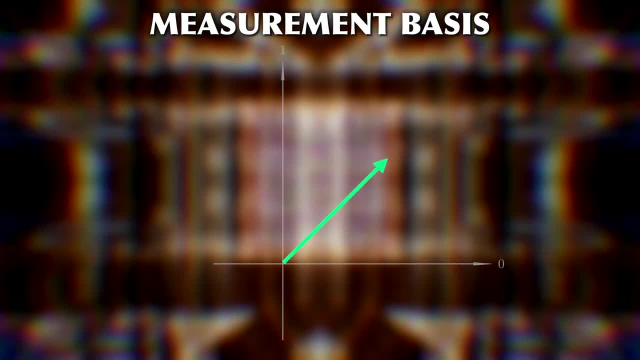 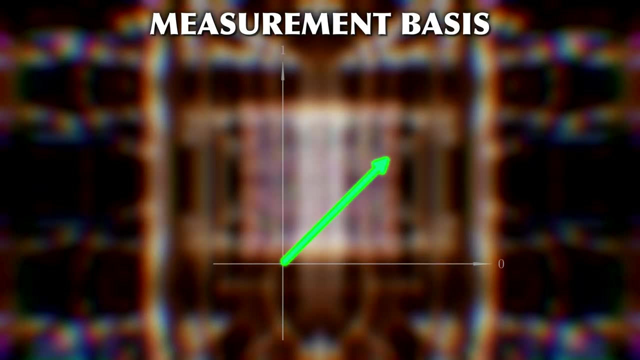 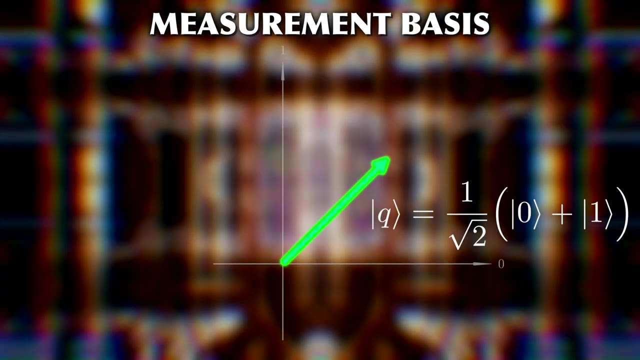 plus one. If we measure it in the C basis, we would get either zero or one each, with a 50% probability. However, if we measure that in the X basis, we will get plus with a 100% probability. After measurement, the state of the qubit will: 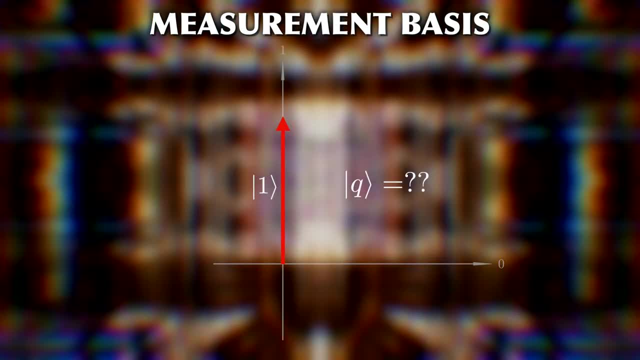 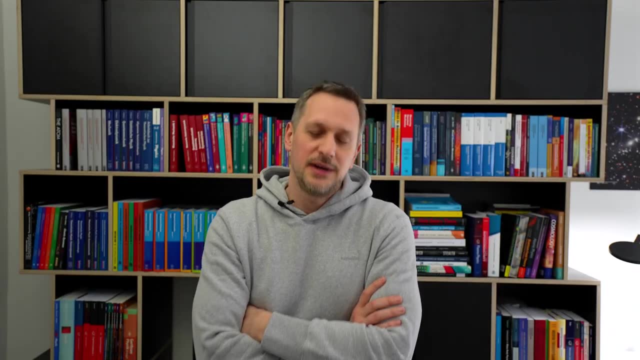 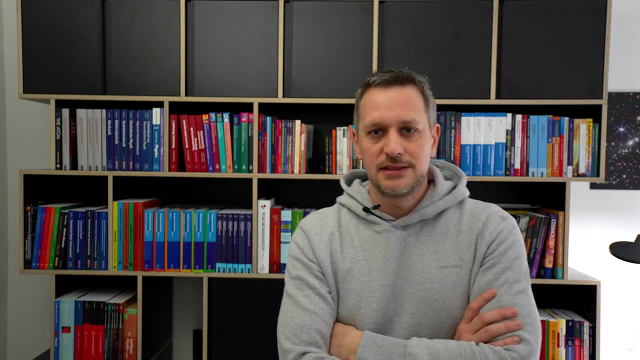 be equal to the measured basis state, and the previous state will be irretrievably lost. These are the rules for measurement, and they are a large part of what makes quantum mechanics so strange. And, to be fair, while we can reasonably well describe the effects of a measurement, there are still many open.